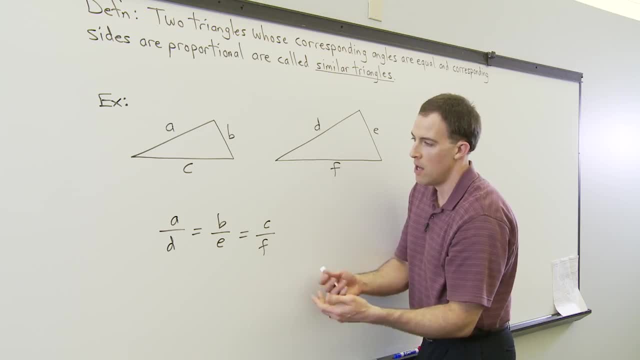 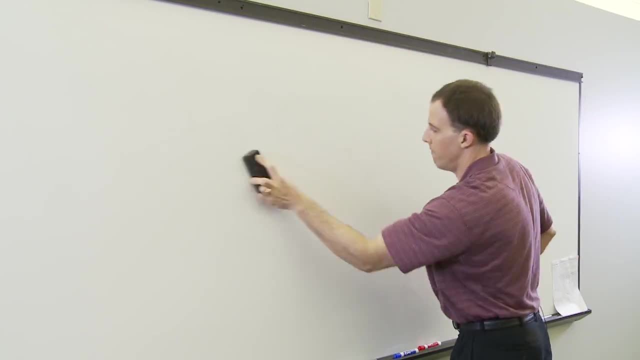 You can take any two of these ratios and set them equal to each other and you have a true proportion. I'm going to do an example right now. In this example, we're given two similar triangles and we're asked to solve for the sides X and Y. 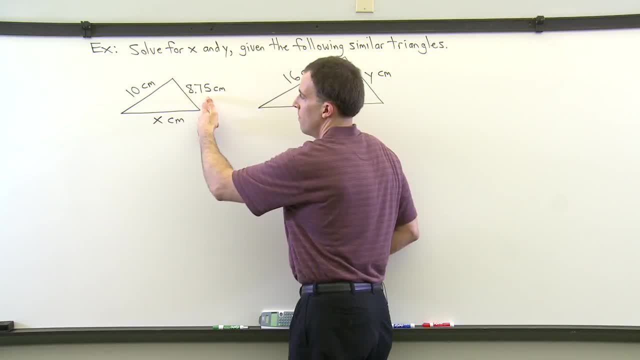 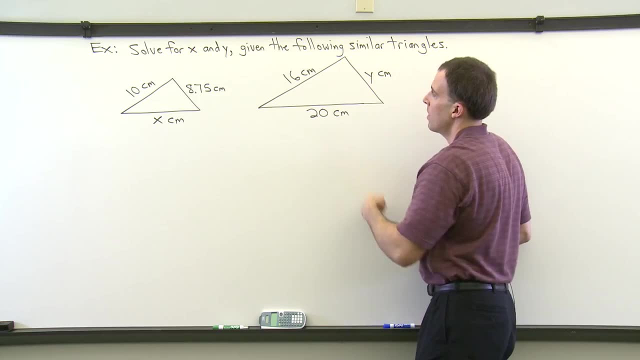 So one of our triangles has sides 10 centimeters, 8.75 centimeters and X centimeters. The triangle that's similar to it has sides 16 centimeters, Y centimeters and 20 centimeters. So first of all, to solve for side X here, side X corresponds with: 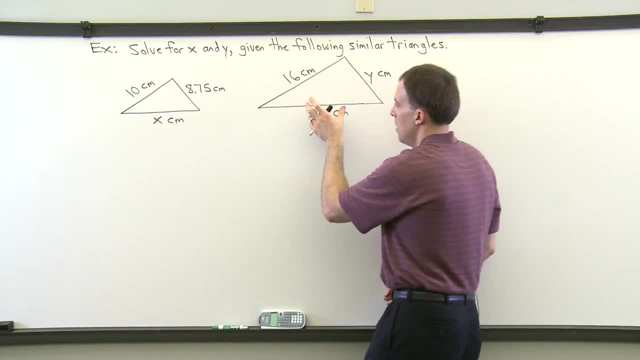 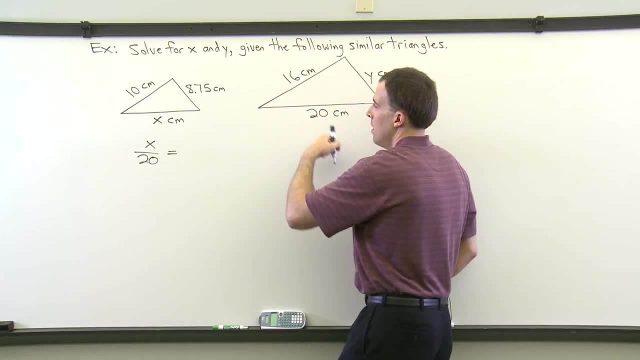 the side, that's 20, in the other triangle. The base of the first triangle is corresponding with the base of the other triangle. So we can set up a proportion- X is to 20, or X over 20 equals- and then we could say 10 is to 16.. 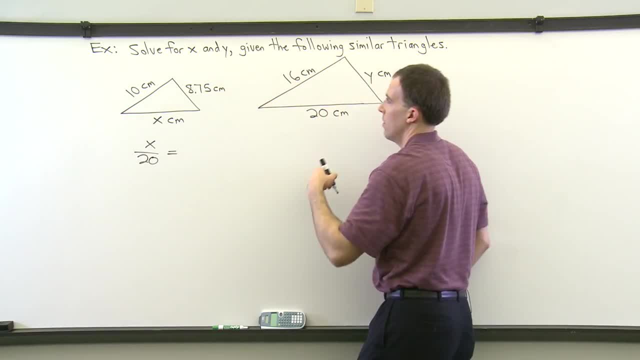 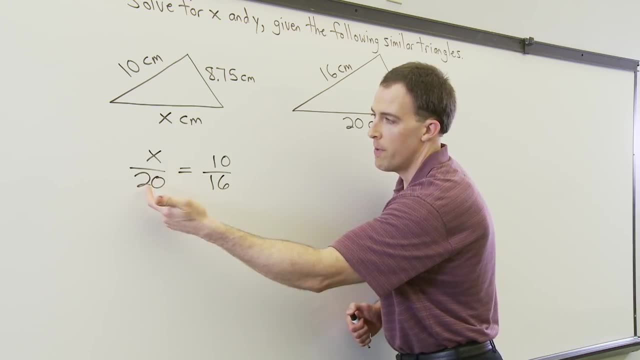 The left side of the smaller triangle is to the right side of the larger triangle, so as 10 is to 16.. And then from there we need to multiply both sides by 20 to isolate X. So we can just take both sides here, multiply by 20.. 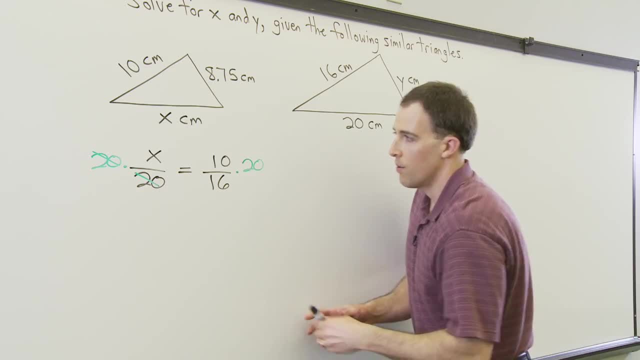 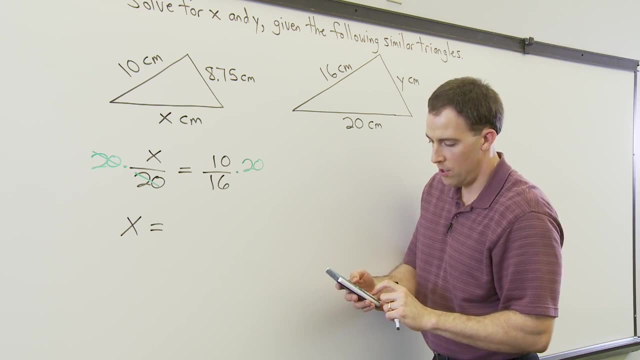 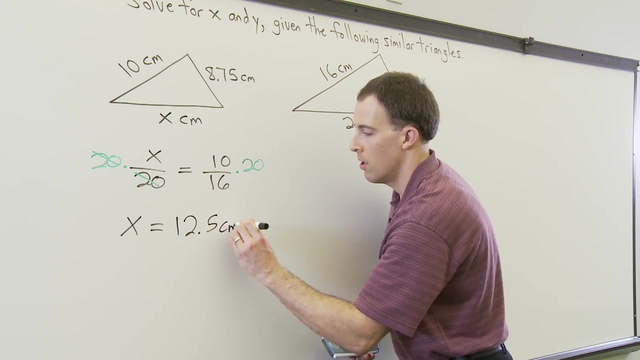 20, and x equals. take your calculator and just take 10 times 20 divided by 16.. So 10, 10 times 20 divided by 16 is 12.5 centimeters. So there's x, The base of the. 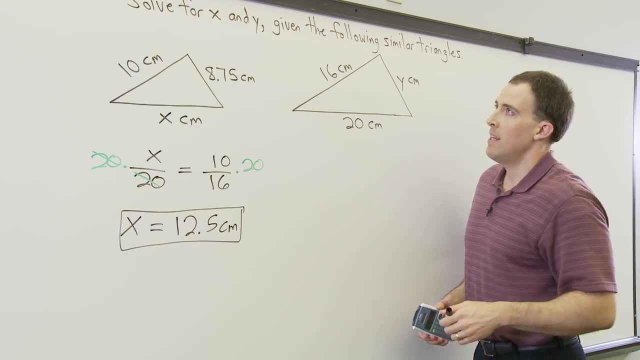 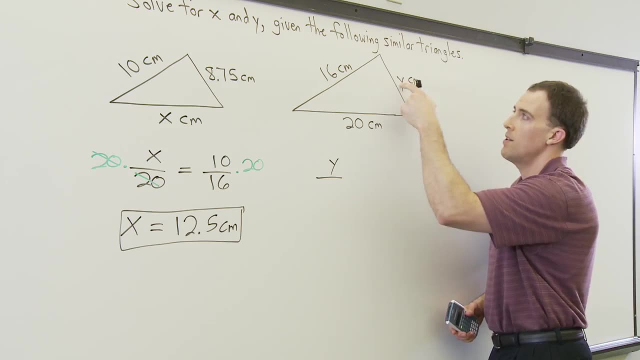 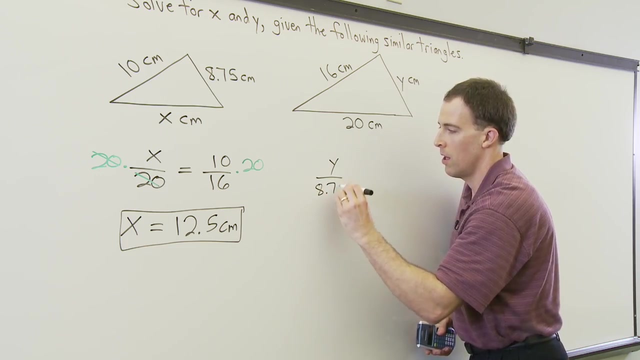 first triangle here is 12.5 centimeters. And then to solve for y, just set up, we need to just set up another proportion involving y. So we could say y is to y is the right side here of the second triangle. We could say y is to 8.75, as, and then we could say: 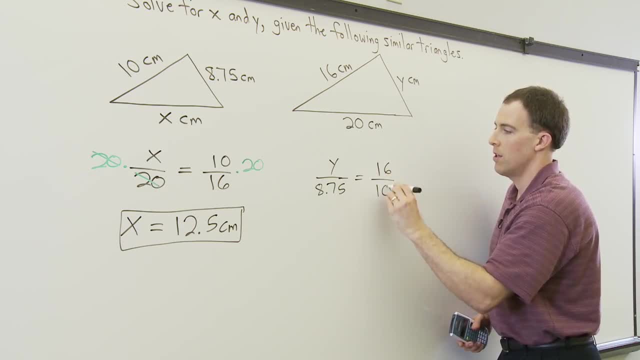 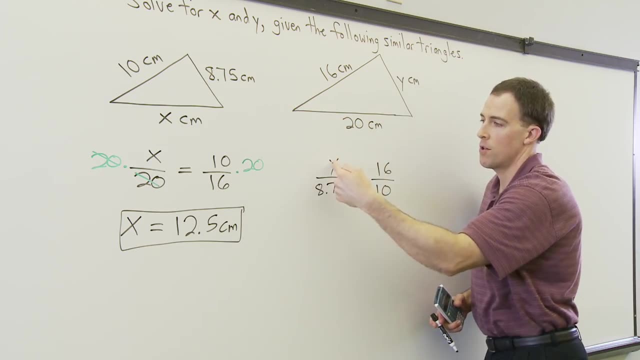 16 is to 10.. The left side of the larger triangle is to the left side of the smaller triangle. So make sure, if you're going from the second triangle to the first triangle in your first ratio, that you go from the second triangle to the first triangle once again in your second. 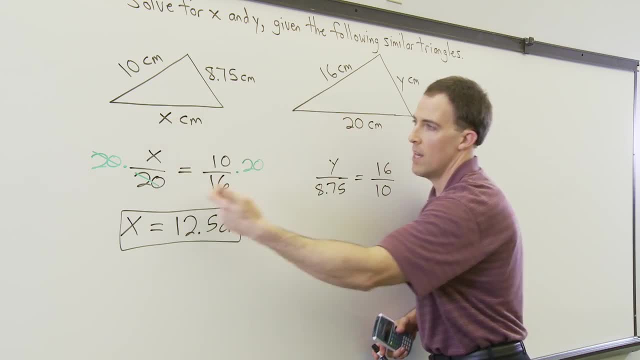 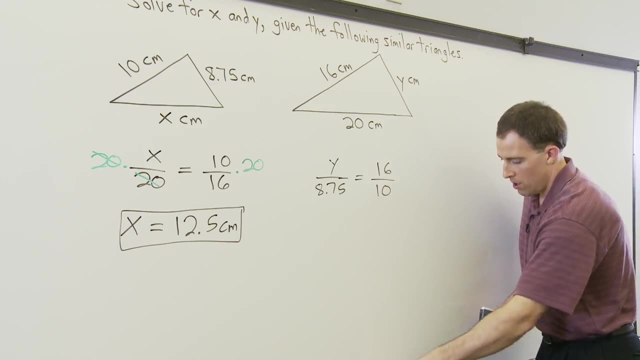 ratio. If you're going from the first triangle to the second one, as we did in solving for x, make sure you go from the first one to the second one in your other ratio there. So to solve this proportion we need to multiply both sides by 8.75.. And that will allow us.